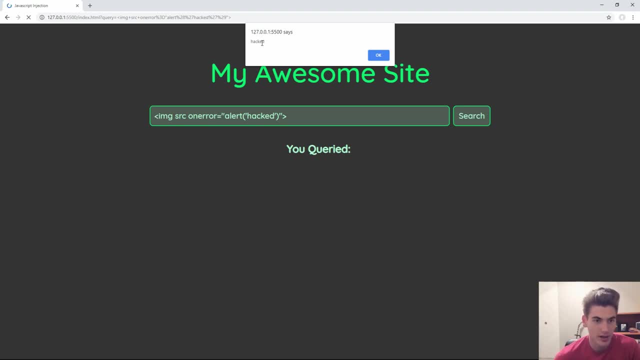 show up in here. So we've essentially injected JavaScript into the page, And now you may be thinking that's not really a problem, because you're just injecting JavaScript into your own page, so the only person you can affect is yourself. But since this query is inside of the 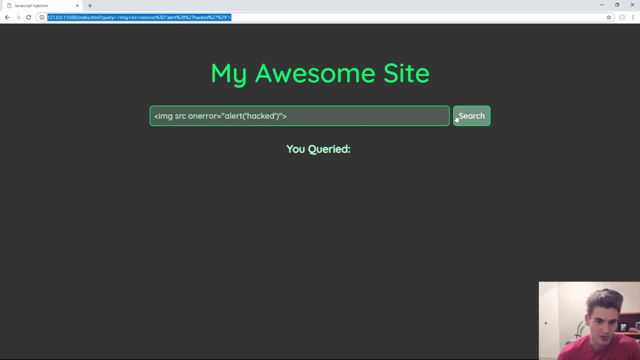 URL here. if I send this URL to somebody, as soon as they go to it, it'll inject this into their page. So, for example, if I go to a new tab here and search this URL, you see that I get this hacked. 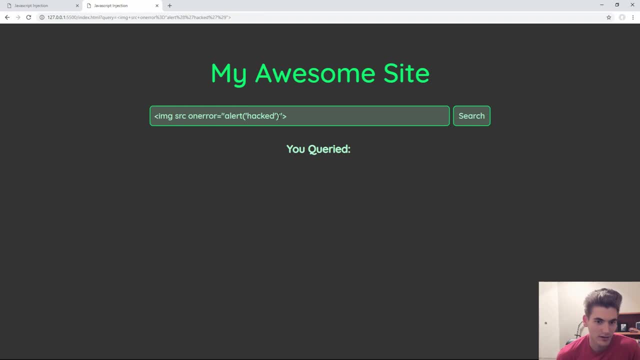 in here and there's a document that I want to do And you may think: well, what can they do with this? They can access some pretty sensitive information. For example, they can access the document cookies. So we'll just go in here with another alert. we'll just say documentcookie. 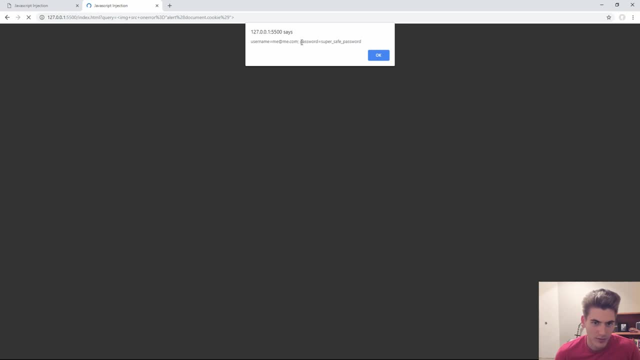 and if we run this again, you can now see that they have access to my username and my password, which are stored in the cookies for this website. Now, in a normal website, they wouldn't actually store your password and username, But they will store a session ID. 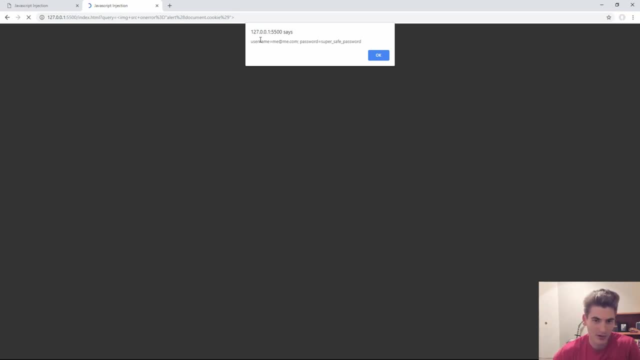 Essentially both your password and username together, and if you have access to that, you can log into the site as that user. So this is something that a hacker could do in order to gain your information, And then all they would have to do inside of their script is just email this or send it to their own site. 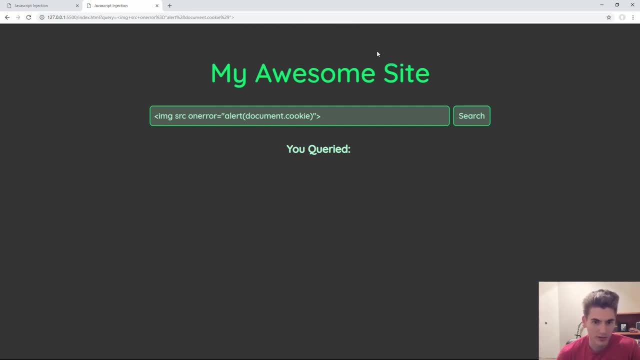 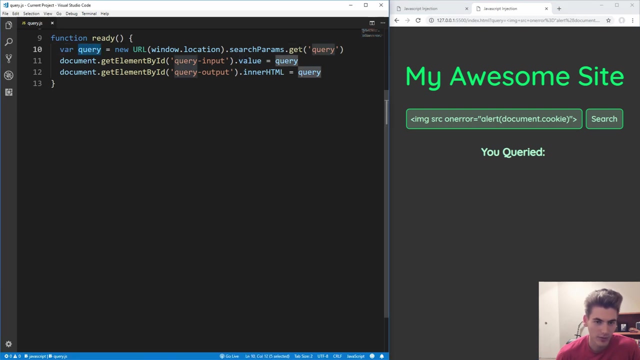 And then they'll have that information Available to themselves just based on this simple JavaScript injection that they're able to perform with this search query. So now let's look at how we can solve this problem. If we look at the actual code for this page here, We see that when our page loads, we get our query from the URL. 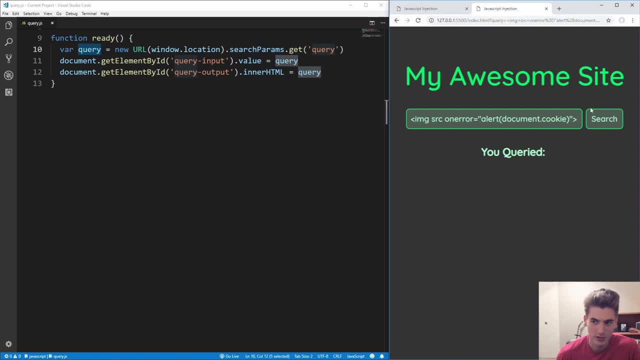 so we get this attribute here that we sent to the page with the search and Then we're setting that to the input so that it's displayed here, And we're also setting it to this query output where it says you queried and then whatever you queried. But we're using inner HTML and inner HTML is not safe to injection if a user inputs valid. 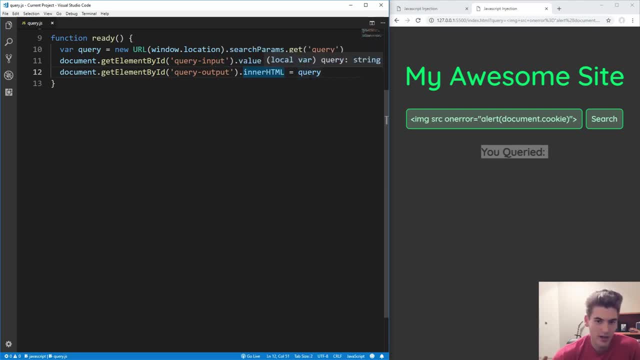 HTML Or a script tag or an image tag, it'll render that as actual HTML instead of as text. In order to get around this, all we need to do is change this to be inner text. Now, if we save that and run, you see that it just shows the text that they put inside of the